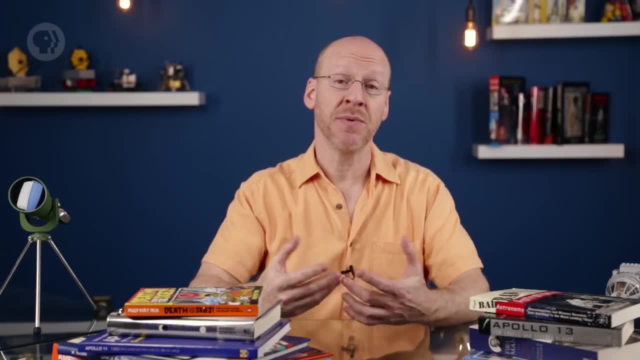 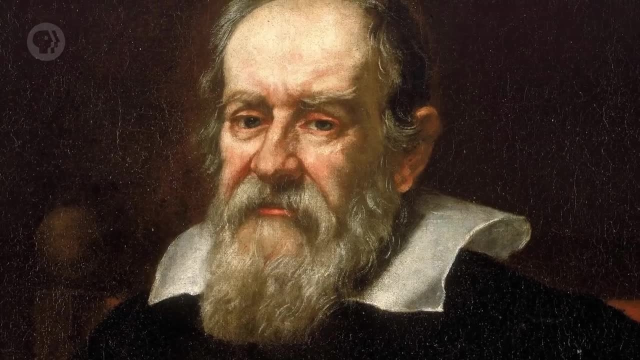 better We can use telescopes. The first person to invent the telescope is lost to history, Despite common knowledge. Galileo did not invent them. He wasn't even the first person to point one at the sky or the first person to publish results, But he was a loud and persistent voice over the 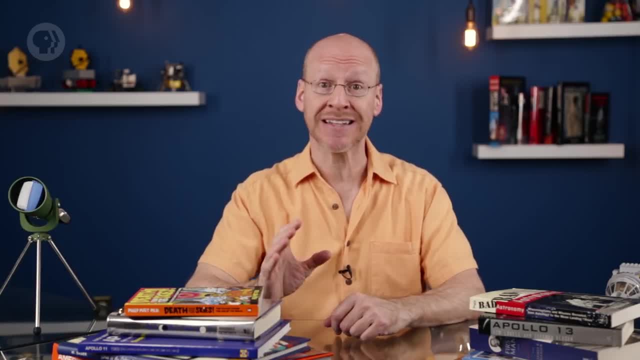 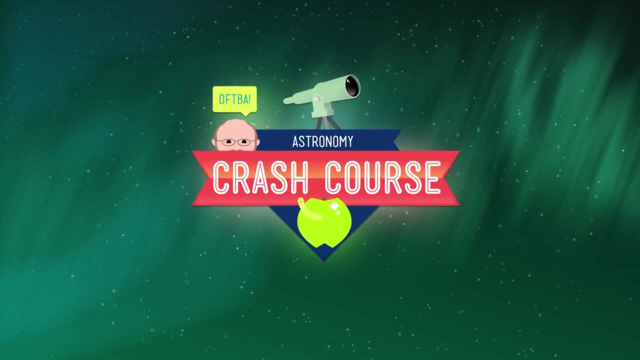 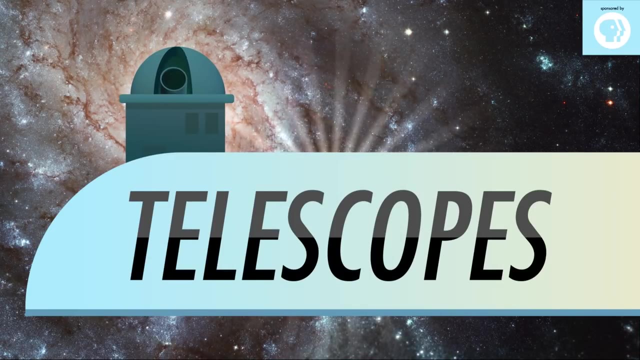 years and his amazing string of discoveries using his crude instrument landed him firmly in the history books. Aggressive self-marketing sometimes pays off. One giant leap for mankind. You might think the purpose of a telescope is to magnify small objects so we can see. 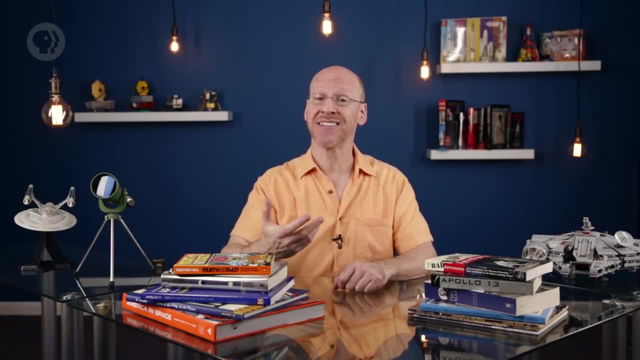 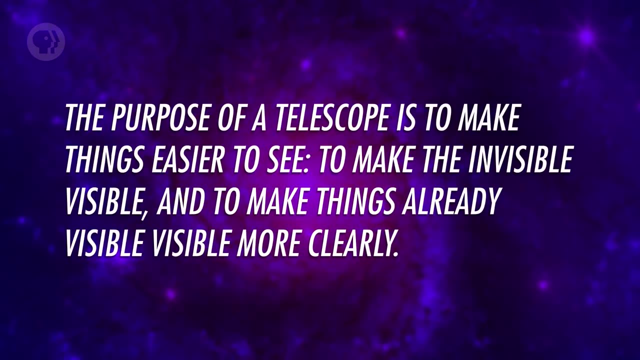 them better. That's how a lot of telescopes are marketed, but, to be honest, they're not exactly the case. If you want to be really general, the purpose of a telescope is to make things easier to see, to make the invisible visible and to make the things already visible. 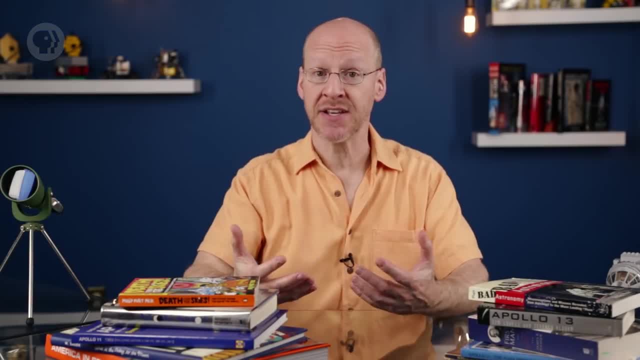 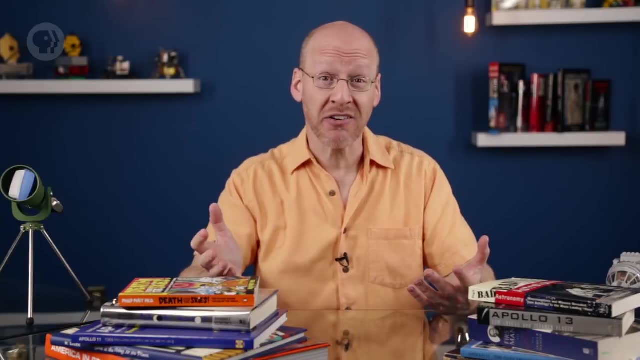 visible more clearly. A telescope works by gathering light. Think of it like a bucket in the rain. The bigger the bucket, the more rain you collect. If your bucket is big enough, you'll get plenty of water, even when it's only sprinkling out. 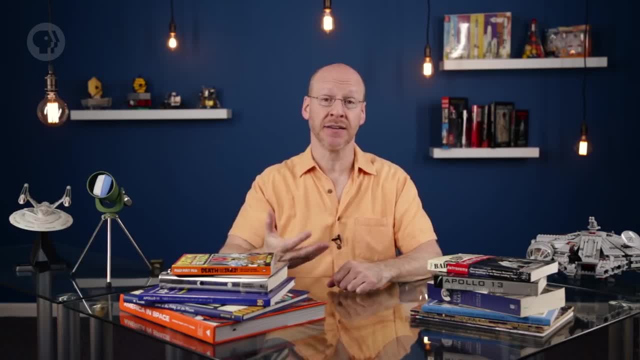 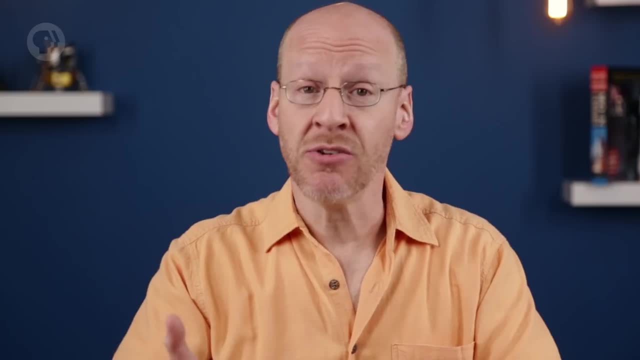 In the case of a telescope, the bucket is an optical device like a lens or a mirror that collects light. We call this device the objective, and the bigger the objective, the more light it collects. Look at your eyes. Well, that's tough. so let's think about our eyes for a moment. 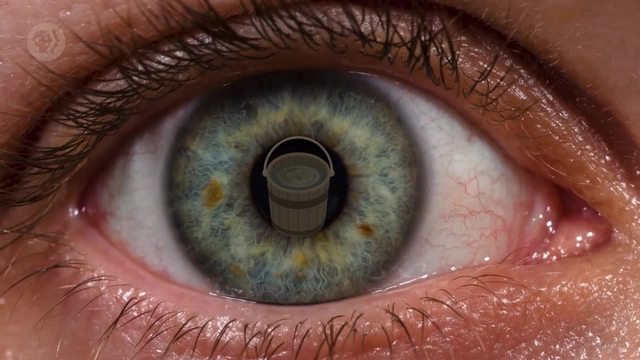 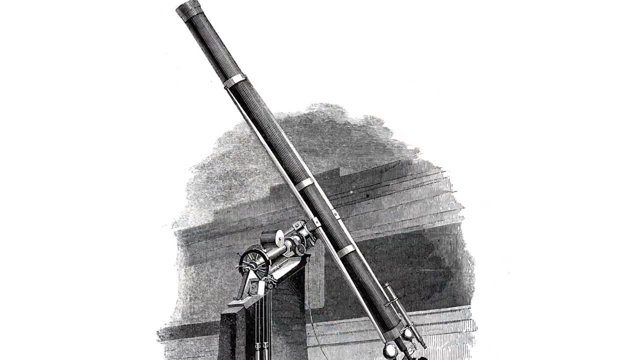 They also work as light buckets, but they only collect light through our pupils which, even under the best of circumstances, are less than a centimeter across- A very tiny bucket indeed. But we can do better. To extend the analogy, a telescope is like a bucket with a funnel. 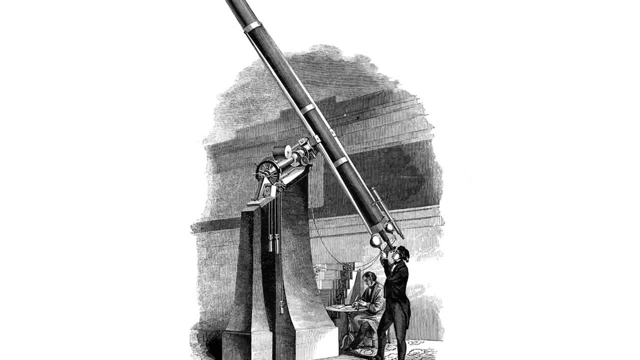 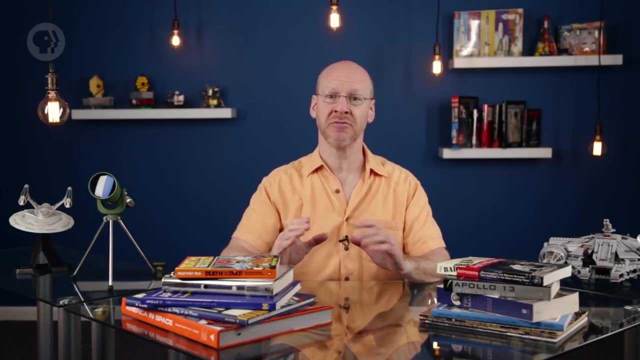 at the bottom. All that light that it collects is then concentrated, focused and sent into your eye. It turns a trickle of light into a torrent. The amount of light it collects depends on the area of the objective. That means if you double the diameter of the collector, you'd collect. 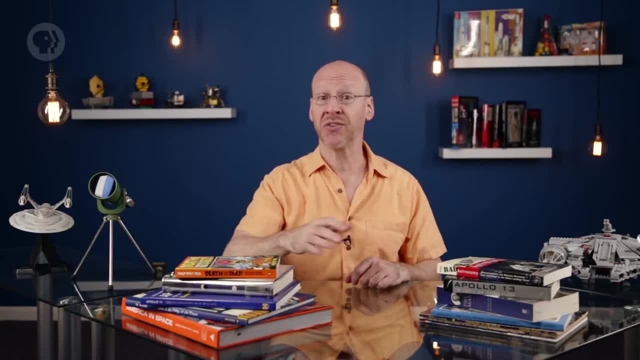 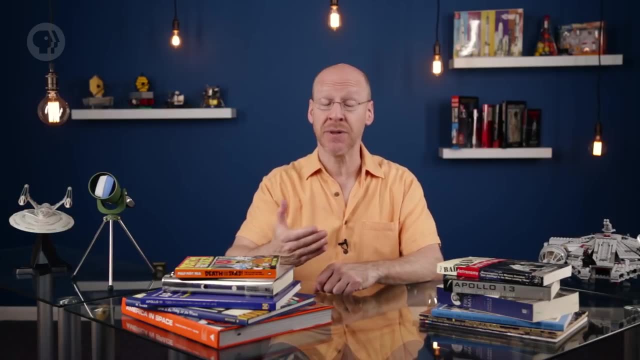 four times as much light because the area of the collector goes up as the square of the radius. Make a bucket ten times wider and you collect a hundred times as much light. Clearly, as telescopes get bigger, their ability to show us faint objects increases enormously. 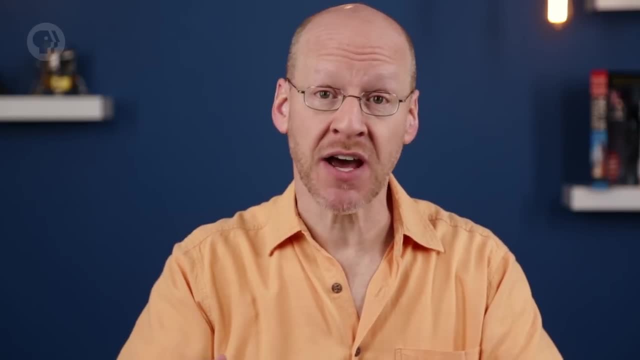 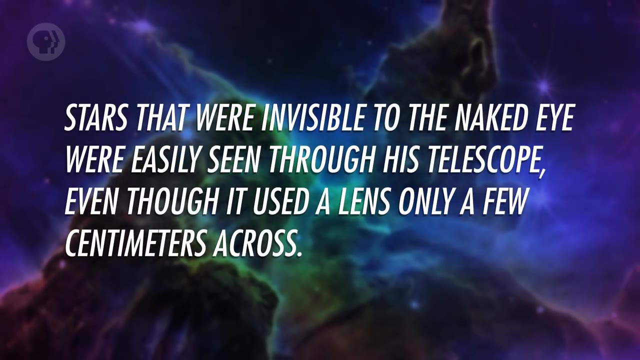 In fact, that was one of Galileo's first and most important discoveries. Stars that were invisible to the naked eye were easily seen through his telescope, even though it only had a lens a few centimeters across. Those faint stars didn't emit enough light for his eyes to see them, but when he 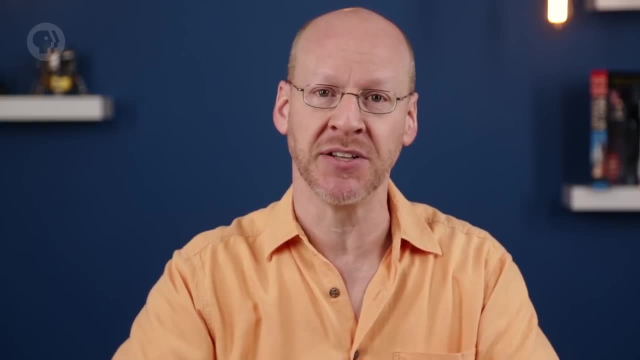 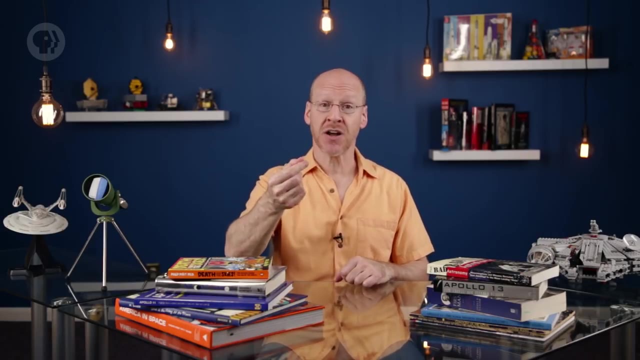 increased his collecting area with a telescope, they popped into visibility. The primary way telescopes work is to change the direction light from an object is travelling. I can see a star with my eye because light from that star is sent in my direction into. 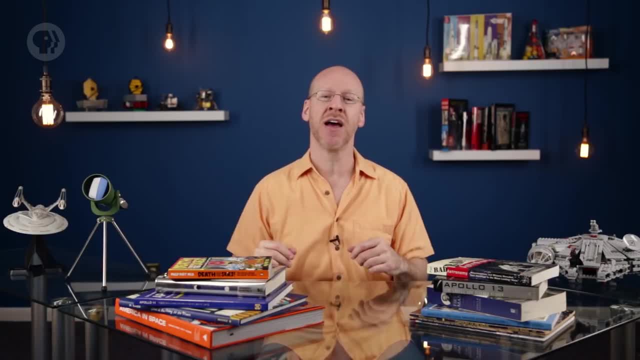 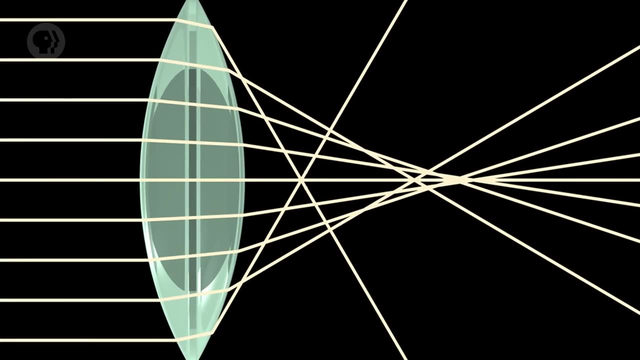 my eye, But most of that light misses my eye, falling to the ground all around me. The telescope collects that light, bounces it around and then channels it in my eye. When the very first telescopes were built, this changing of the direction of light was 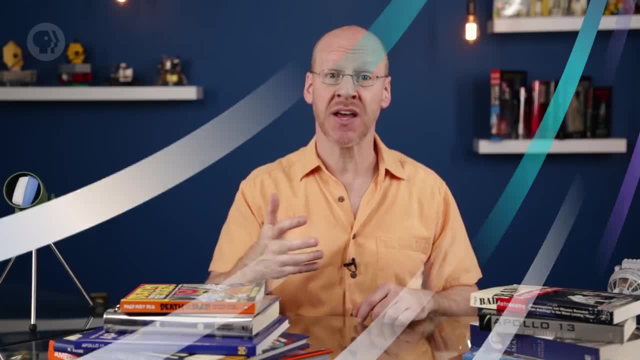 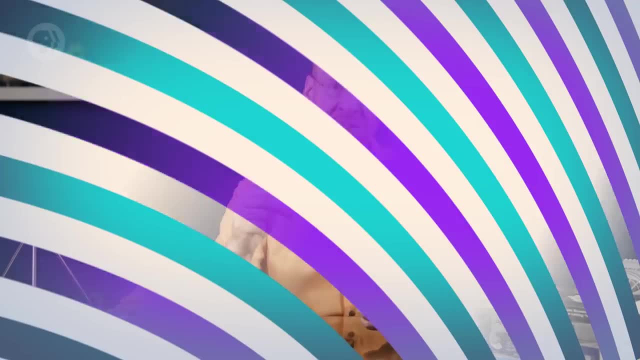 done using lenses When light was coming into your eyes. it was very important that the light goes from one medium to another — say from going through air to going through water or glass — it changes direction slightly. You see this all the time. A spoon sitting. 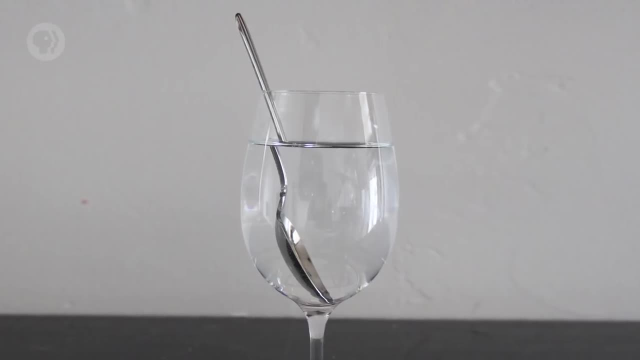 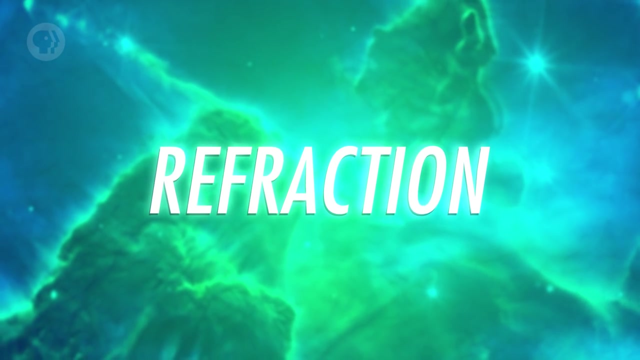 in a glass of water looks bent or broken. The spoon is doing just fine, but the light you see from it is getting bent, distorting the image. This bending is called refraction. The way light bends depends on what's bending it- like water or glass, and the shape of 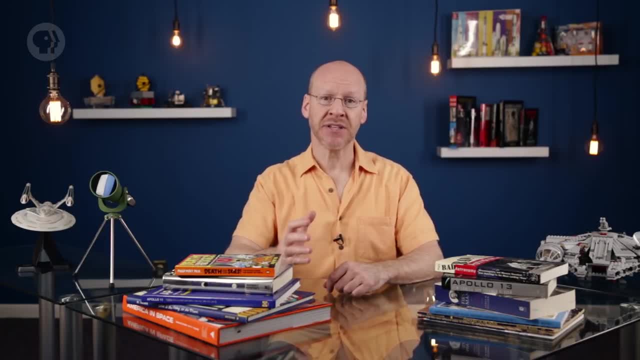 the object doing the bending. It so happens that if you grind a piece of glass into a lens shape, it bends — or refracts — the incoming light in a cone, focusing it into a single spot: It's a light funnel. This refraction has a couple of interesting results. For one thing, the light from the 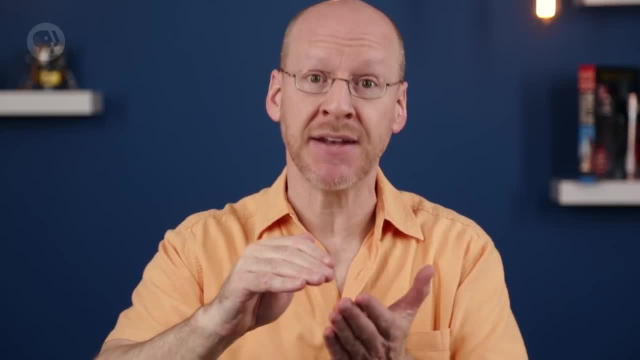 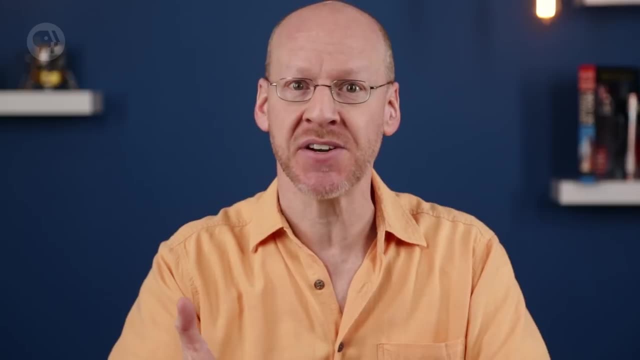 top of a distant object is bent down and the light from the bottom is bent up. When this light comes to a focus, it means you see the object upside down. It also flips left and right, which can be a little disconcerting and takes getting used to when you're using 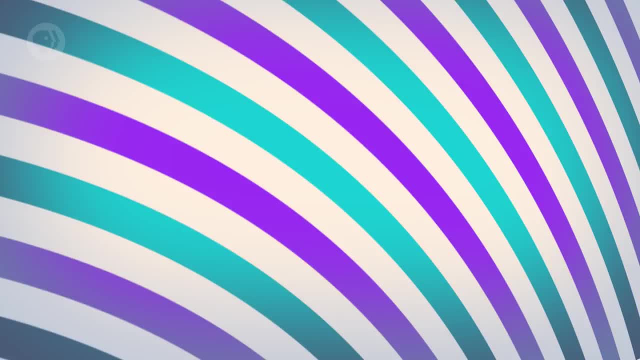 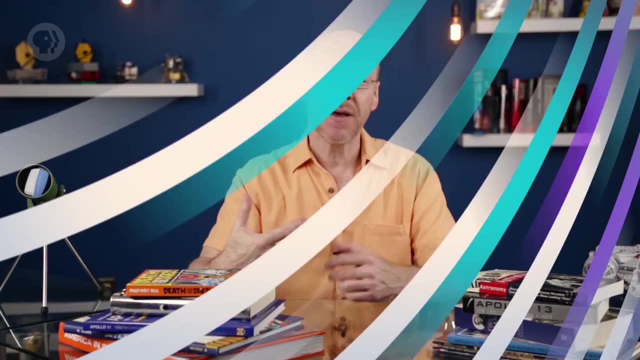 a refracting telescope. For another thing: the lens can magnify the image. That's again because the light is bent And the image created of an observed object can appear larger than the object does by eye. It depends on a lot of factors, including the shape of the lens, the distance to the 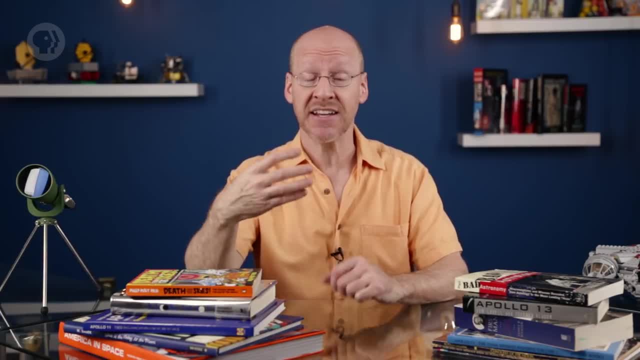 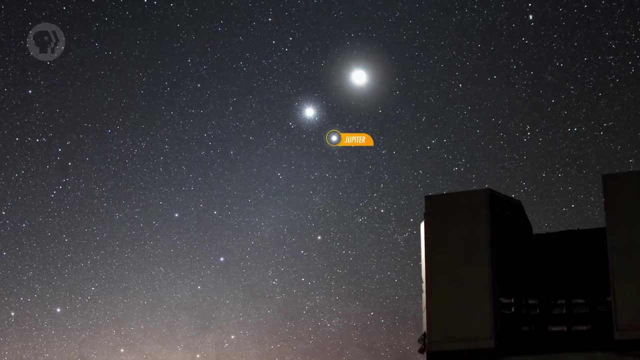 object and how far away the lens is, But in the end what you get is an image that looks bigger. That has obvious advantages. A planet like Jupiter is too far away to see as anything other than a dot to the eye, But a telescope makes it appear bigger and details can then. 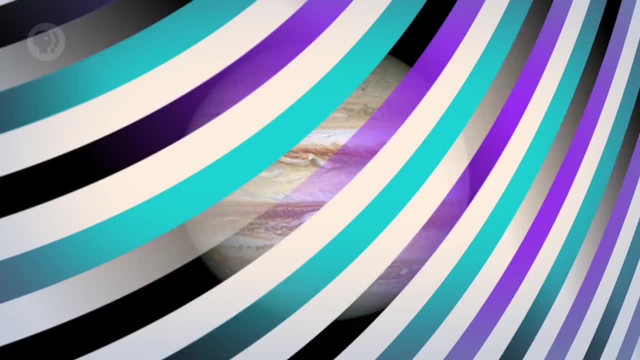 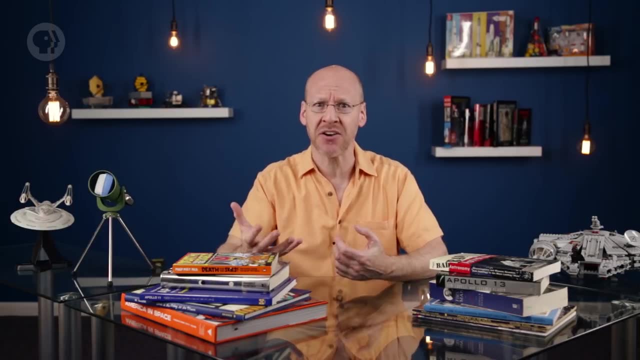 be seen When Galileo and other early astronomers pointed their telescopes at the sky. multitudes were revealed: Craters on the Moon, The phases of Venus, Jupiter's moons, The rings of Saturn And so much more. The universe itself came into focus. 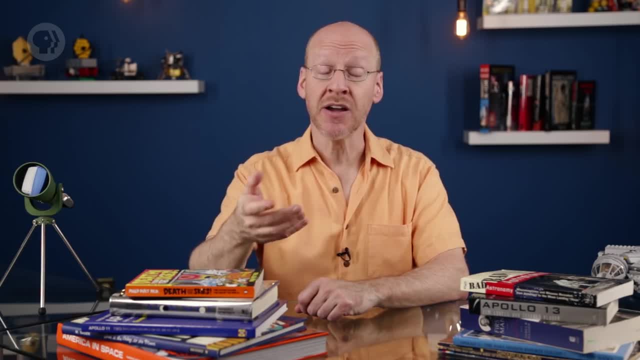 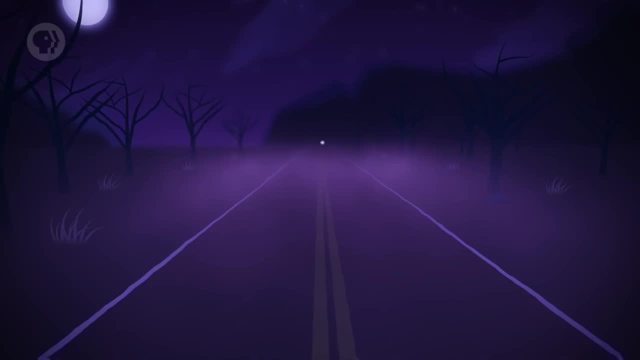 When astronomers talk about using a telescope to make details more clear, they use a term called resolution. This is the ability to separate two objects that are very close together. You're familiar with this When you're driving on a road at night, a distant car coming toward. 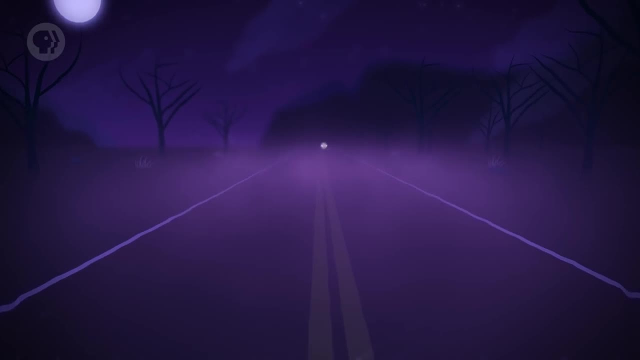 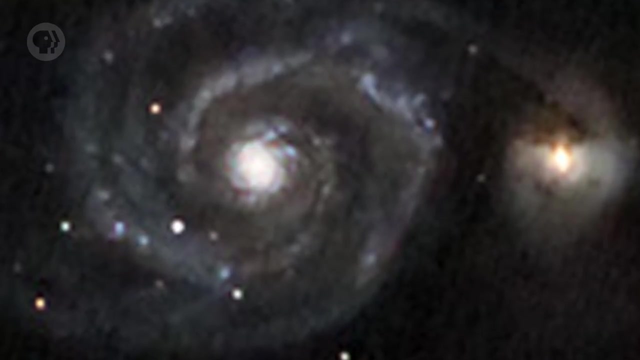 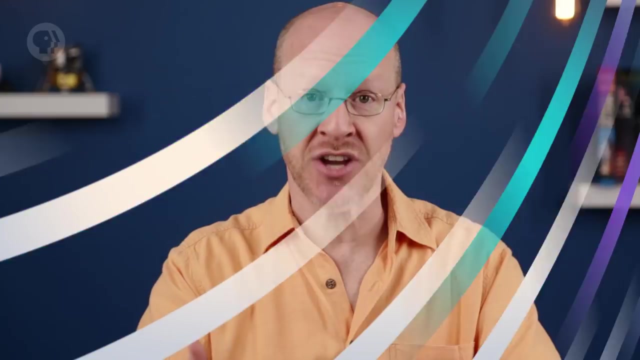 you appears as a single light. When it gets closer the light separates out, resolves into two headlights. A telescope increases resolution, making it easier to say, look at two stars close together or see details on the Moon's surface. The resolution depends in part on the size of the objective. In general, the bigger the 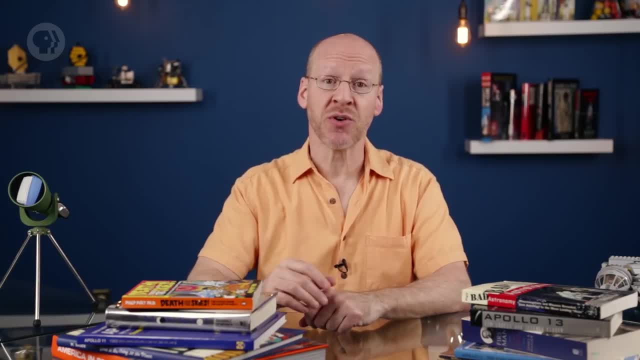 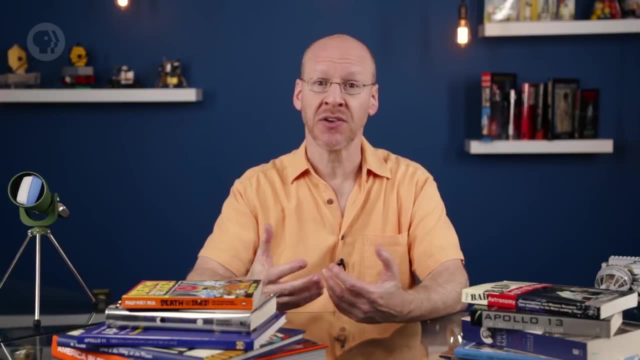 telescope objective, the better your resolution is. Resolution is more useful than magnification when talking telescopes. Fundamentally, there's a limit to how well your telescope resolves two objects, But there's no limit to how much you can magnify the image. If you magnify the image beyond what the telescope can actually. 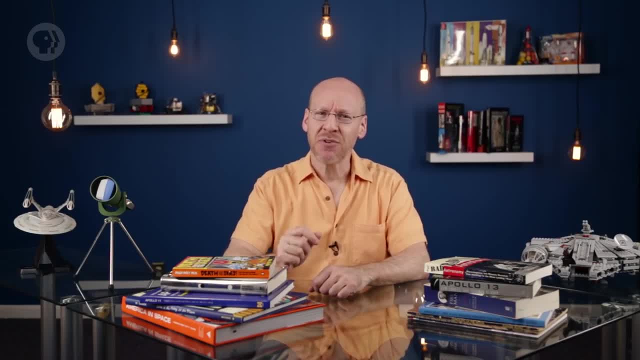 resolve, you just get mush. Refracting telescopes are great But they suffer from some problems. For instance, if you have a telescope that is too big for the telescope, you can just put it in the right, But they suffer from a big problem. Big lenses are hard to make. They get thin near the edge. 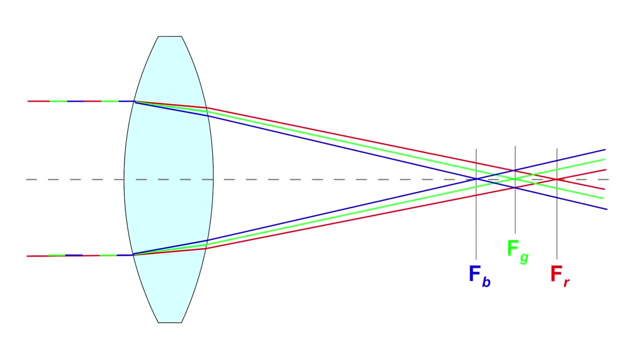 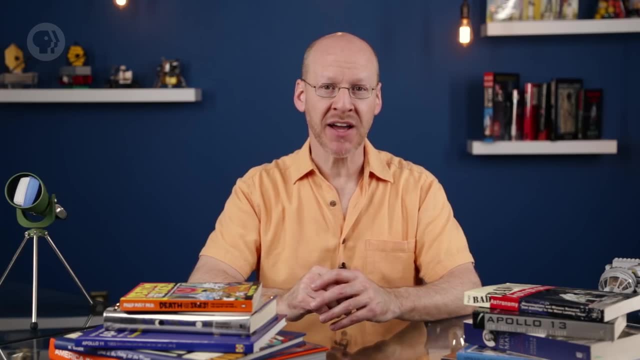 and break easily. Also, different colors of light bend by different amounts as they pass through the lens. So you might focus a red star, say, and a blue one will still look fuzzy. No less of mind than Isaac Newton figured a way around this: Use mirrors- Mirrors also. 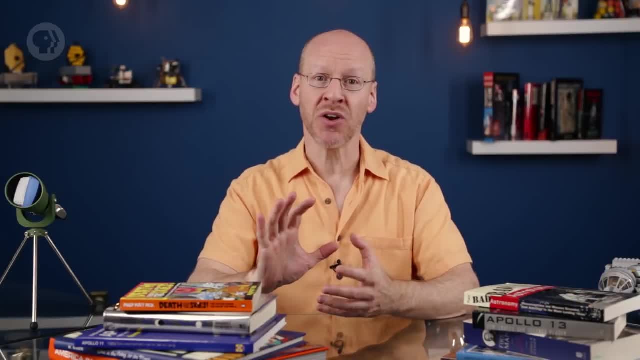 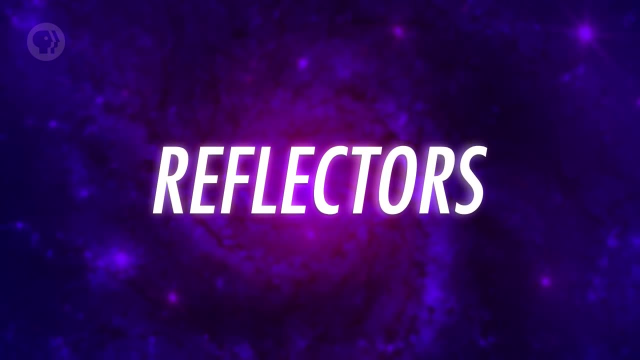 change the direction light travels And if you used a curved mirror, you can also bring light rays to a focus. Telescopes that use mirrors are called reflectors. The advantages of reflectors are huge. You only have to polish one side of a mirror. 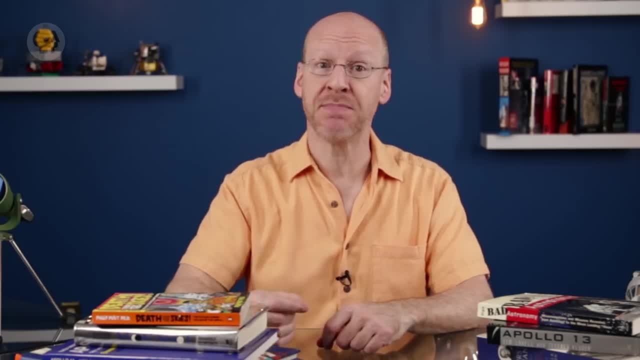 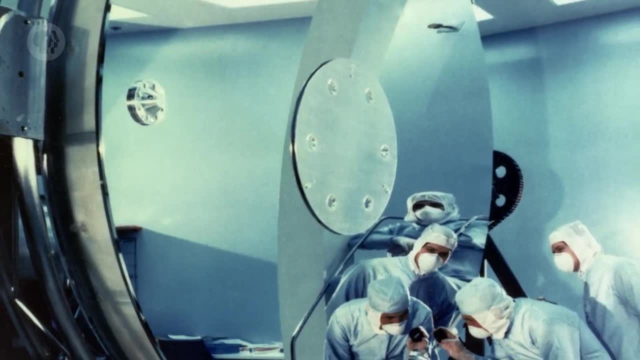 where a lens has two sides. Also, a mirror can be supported along its back, so they can be manufactured much larger, more easily and for less money. Although there have been many improvements made over the centuries, most big modern telescopes at their heart are based on the Newtonian design And, in fact, no large professional-grade. 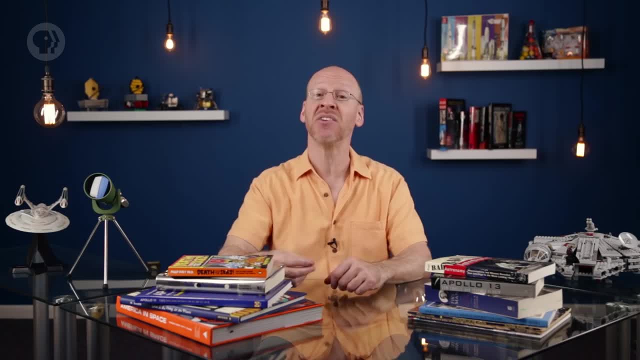 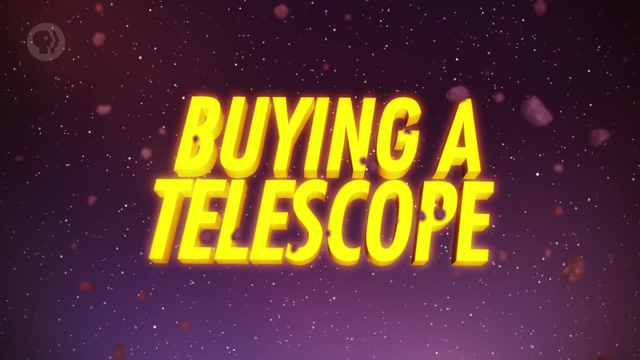 telescopes made today have a lens as their objective. Nowadays, it's all done with mirrors. And that brings us to this week's aptly named Focus On. The most common question I'm asked is: what is a focus on Besides, hey, who does your hair Is? hey, Phil, what kind of telescope should I buy? It's a legitimate question, but it's very difficult to answer. Imagine someone walked up to you and asked: what kind of car should I buy? That's impossible to answer without a lot more information. Same for telescopes: Do you want to look at the Moon and planets, Or are fainter more? 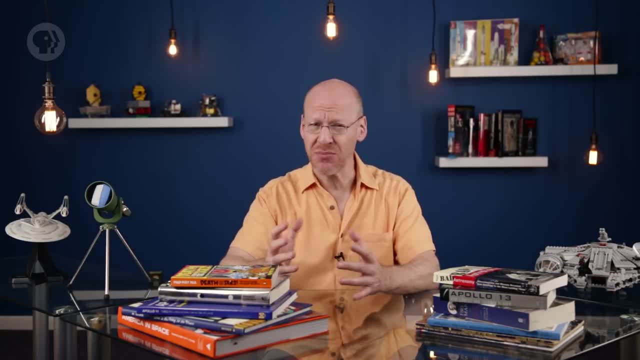 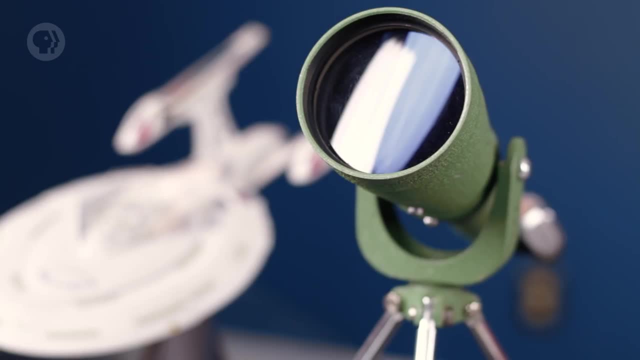 difficult-to-spot galaxies. Are you really devoted to this Or is it more of a pastime? Is this for a child or an adult? These questions are critical. Most small scopes are refractors, which are good for looking at detail on the Moon and planet. 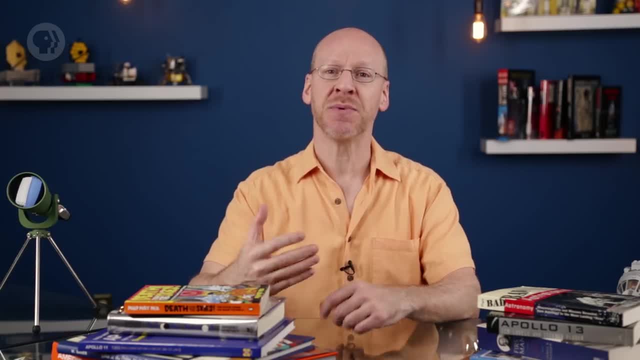 They tend to magnify the image more than reflectors do, But they're tricky to use because they flip the image left and right and up and down. Bigger scopes are good for fainter objects but are more expensive and can be difficult. 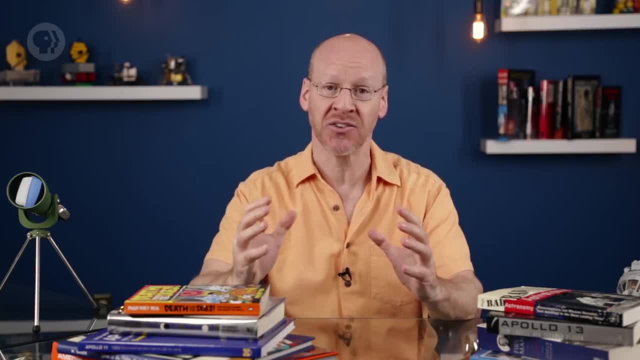 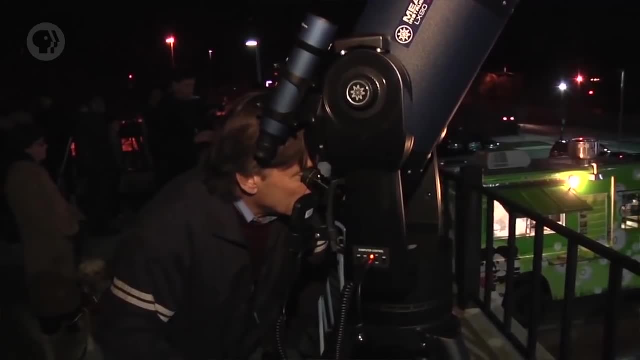 to set up and use. I hate hearing about a scope that just collects dust because it was bought in haste. So here's what I recommend: Find an observatory, planetarium or local astronomy club. They're likely to have star parties, public observing events where you can look at and through. 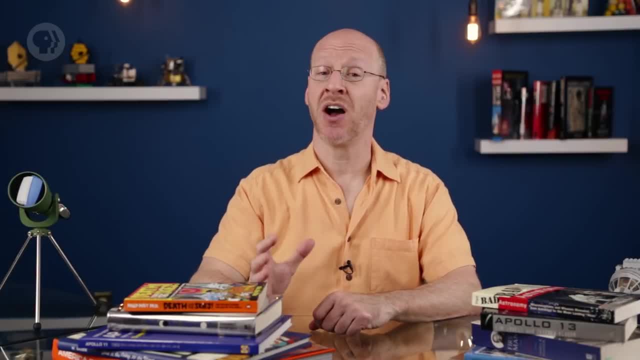 different kinds of telescopes. Their owners are almost universally thrilled to talk about them. As an astronomer, I can assure you that the problem with astronomers isn't getting them to talk. it's shutting them up. So you'll get lots of great first-hand advice. 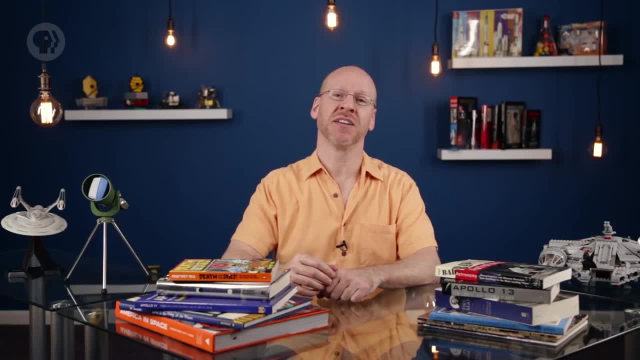 and experience. Also, I usually recommend getting binoculars before a telescope. They're easy to use, fun to use, easy to carry around and you can get good ones for less money and still see some nice things, Even if you decide not to get more into astronomy as a hobby. they can also be used during the 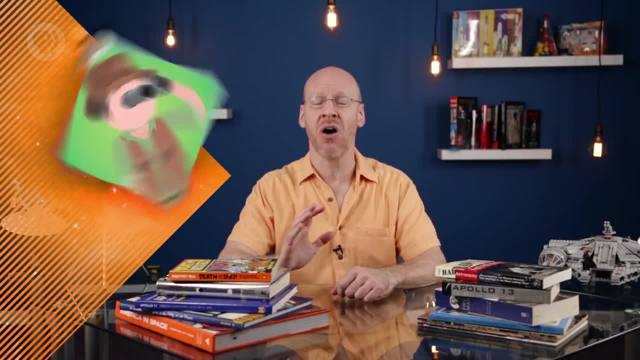 day on hikes and for birdwatching. I have a couple of pair of binoculars and I use them all the time. There's a third aspect of telescopes that's very important: Beardwatching. There's a third aspect of telescopes that's very important: Beardwatching. 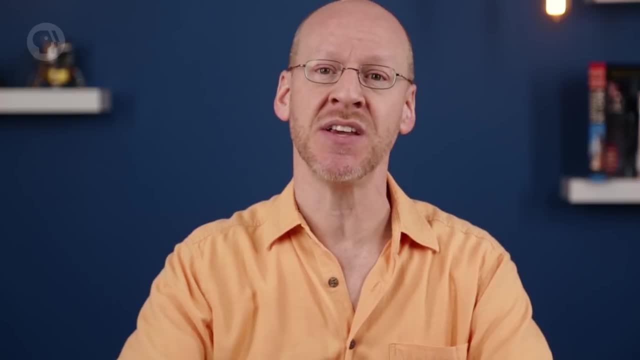 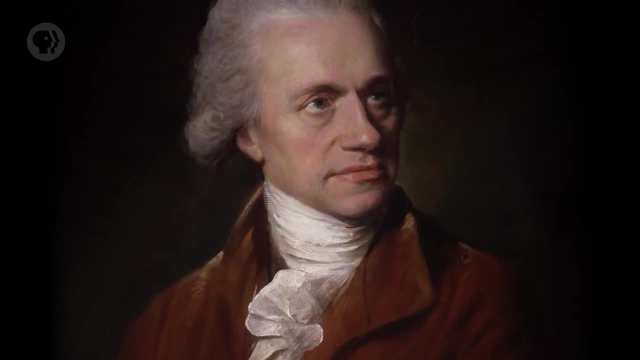 Beardwatching. They're beyond resolution and making faint things easier to see. They can literally show us objects outside of the range of colors our eyes can see. In the year 1800, William Herschel discovered infrared light, a kind of light invisible. 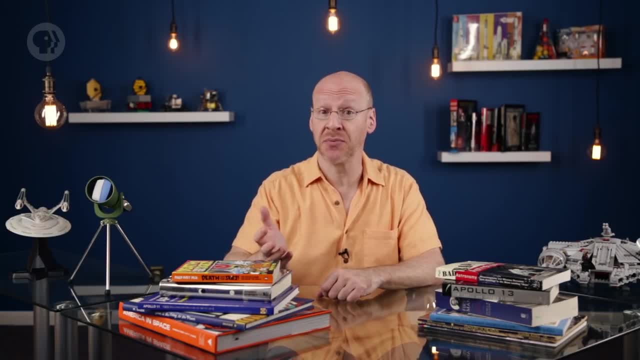 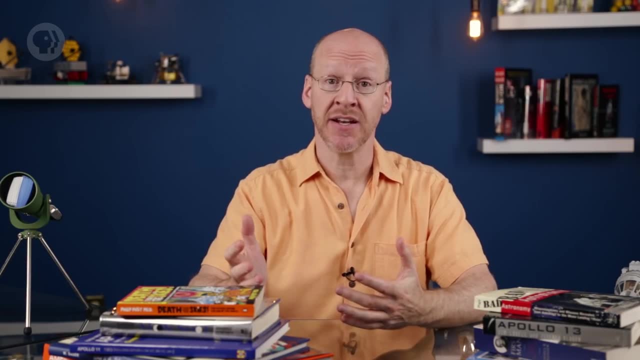 to our eyes In the time, since we've learned of other forms of invisible light: Radio, microwave, ultraviolet X-rays and gamma rays. Astronomical objects can be observed in all these flavors of light if we have telescopes. 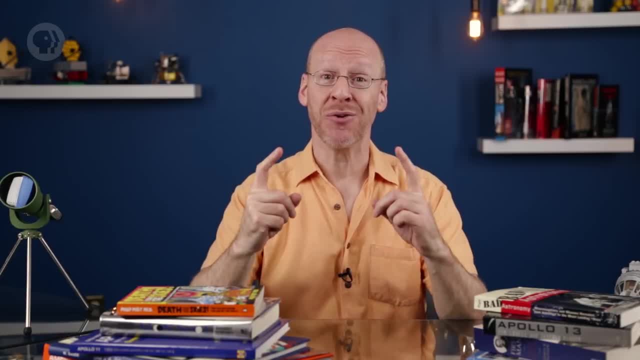 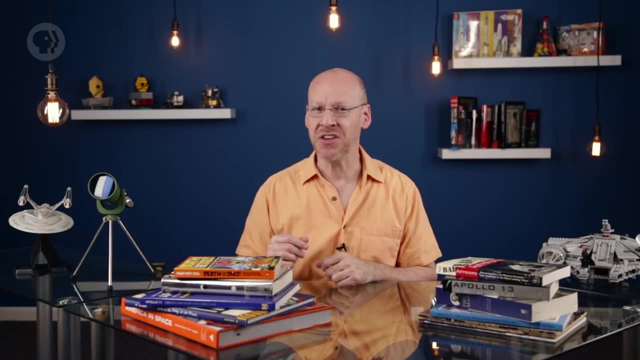 that are designed to detect these flavors of light. Radio waves pass right around normal telescopes, ones that we use to observe visible light. X-rays and gamma rays pass right through them as if they aren't even there. But we're smart, we humans. We learned that giant metal dishes can and will bend radio. 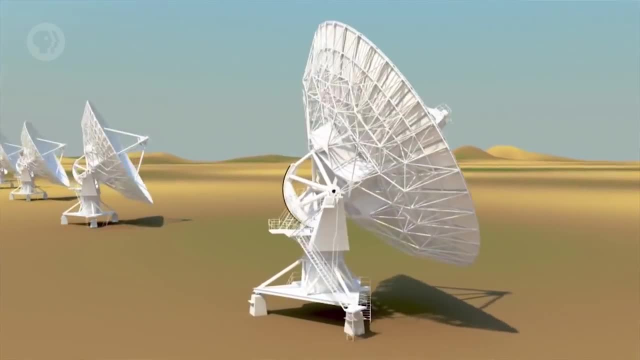 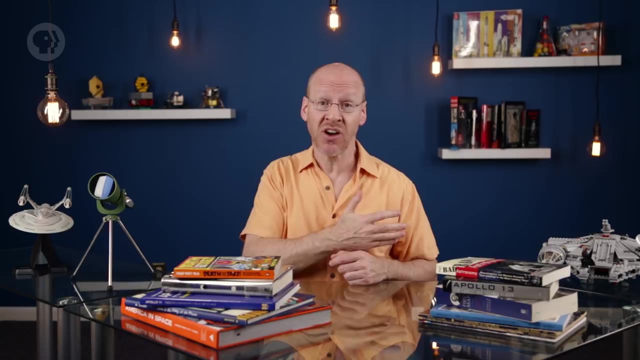 waves and can be formed just like gigantic Newtonian mirrored telescopes. In fact, different forms of light need different kinds of telescopes, and once we've figured out how we've built them, We can now detect cosmic phenomena across the entire spectrum of light from radio waves. 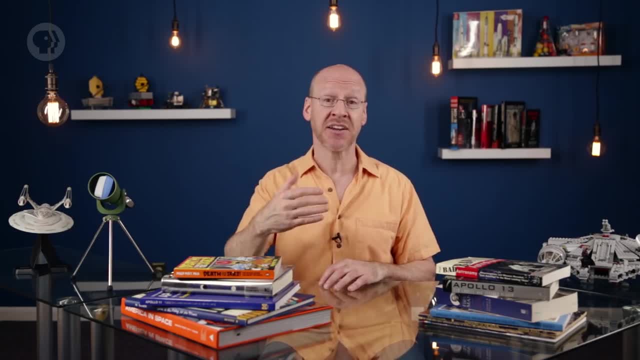 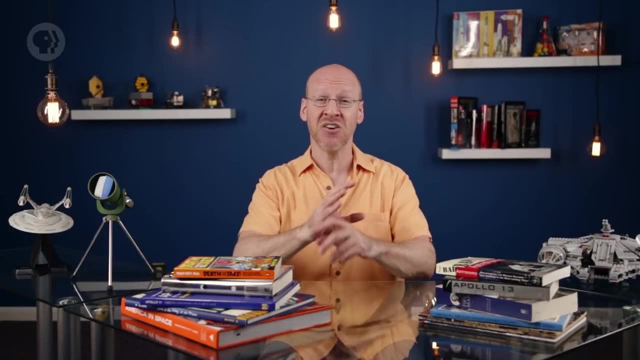 to gamma rays, and have even built unconventional telescopes that detect subatomic particles from space as well, such as neutrinos and cosmic rays. Because of this, we can now detect cosmic phenomena. Because of this, we've learned far more about the universe than Galileo could have imagined. 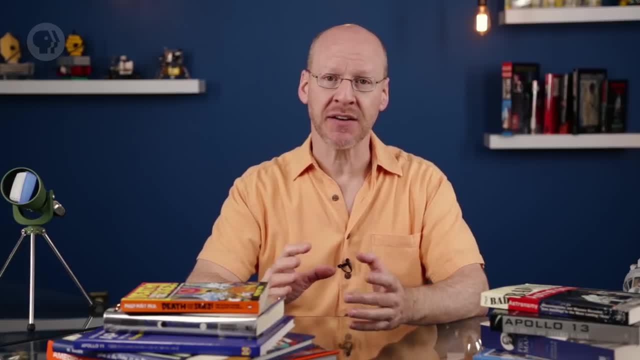 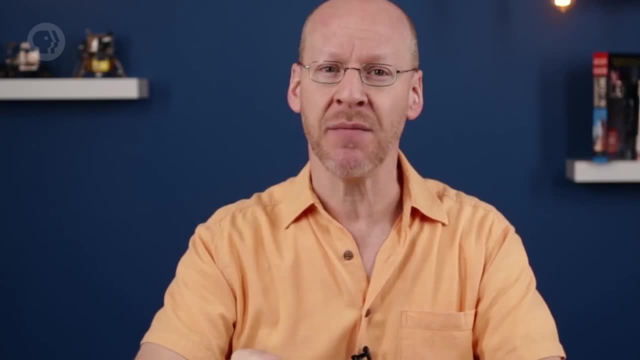 And we're in the midst of another revolution too. The actual biophysics is complicated, but in a sense, our eyes act like movie cameras, taking pictures at a frame rate of about 14 images per second. That's a short amount of time. Photographs, though, can take far. 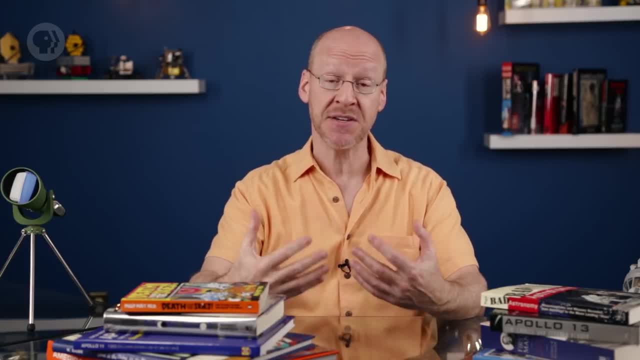 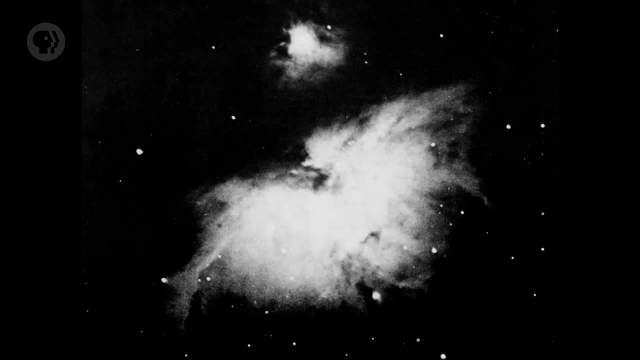 longer exposures allowing the light to build up, allowing us to see much fainter objects. The first photographs taken through a telescope were done in the 1800s. This has led to innumerable discoveries. For example, in the 20th century, giant telescopes with giant telescopes were 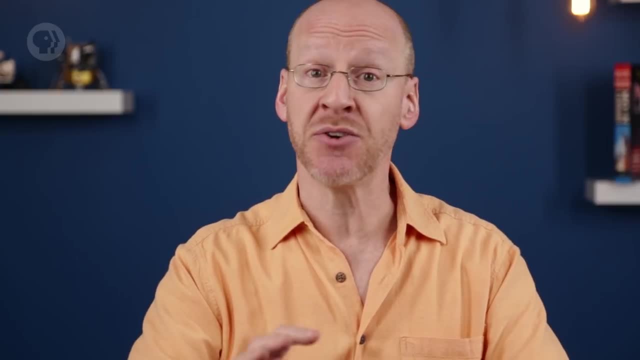 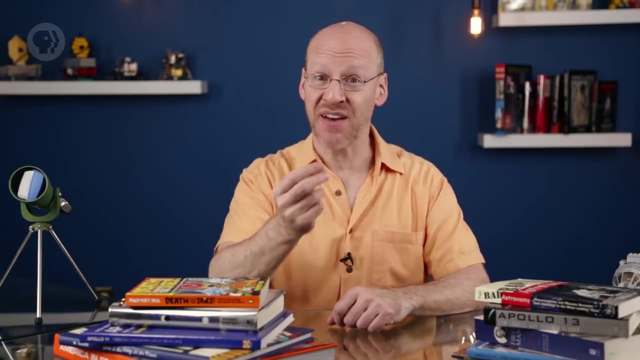 used. Photographs with giant cameras reveal details in distant galaxies that led to our understanding that the universe is expanding- a critically important concept that we'll dive into later in the series. And now we have digital detectors, similar to the ones in your phone camera, but far. 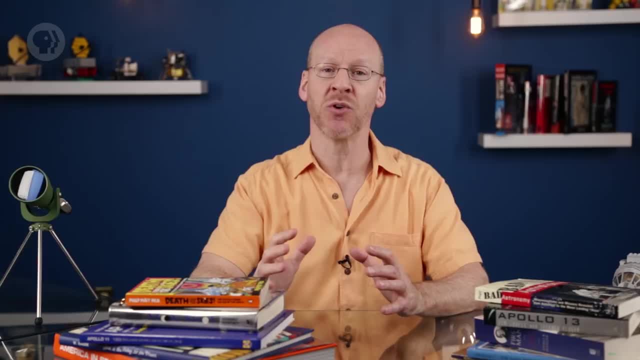 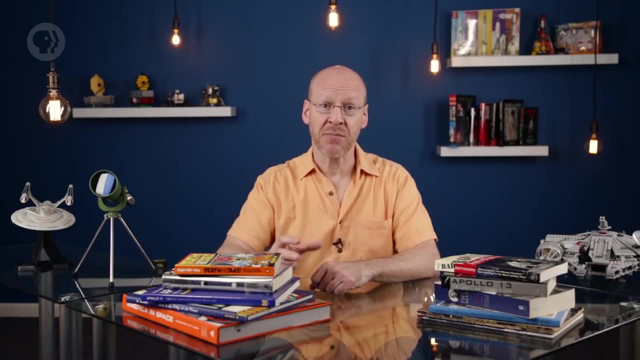 larger and far more sensitive. They can be dozens of times more light-sensitive than film, able to detect in minutes objects that would have taken hours or more to see using film. These digital cameras can also be designed to detect ultraviolet light, infrared and. 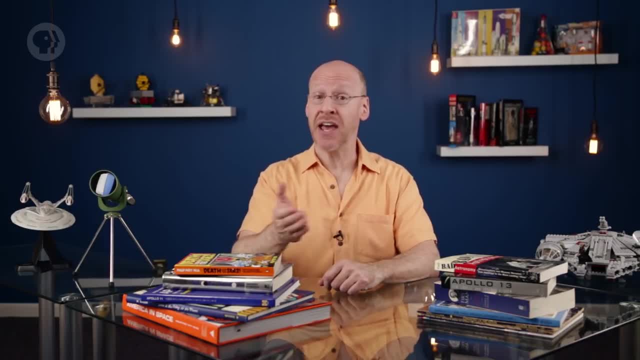 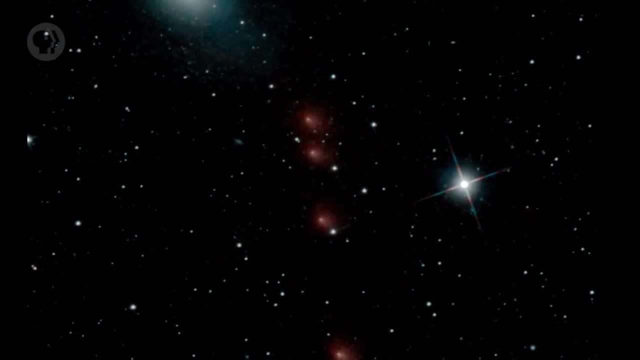 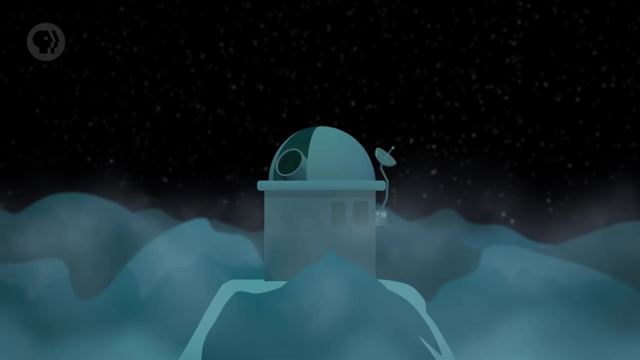 more. They can bounce of that data easily on computers and use those computers to analyze that huge ocean of information, performing tasks too tedious for humans. Most asteroids and comets are discovered using autonomous software, for example, looking for moving objects among the tens or hundreds of thousands of fixed stars in digital images. 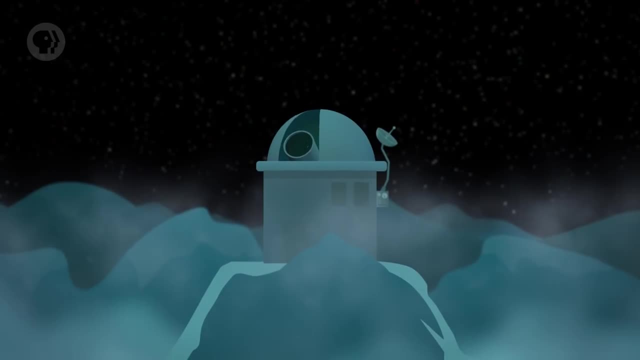 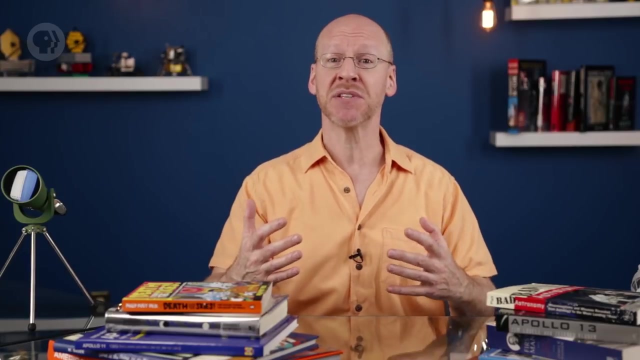 This is also ushered in the era of remote astronomy. A telescope can be on a distant mountain and programmed to scan the sky automatically. It also means we can loft telescopes into space above the sea of air in our atmosphere that blurs and distorts distant, faint objects. 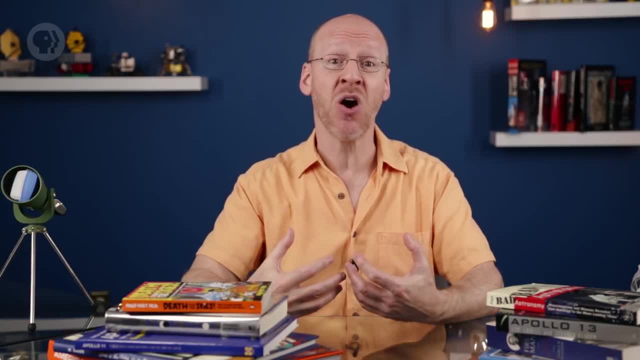 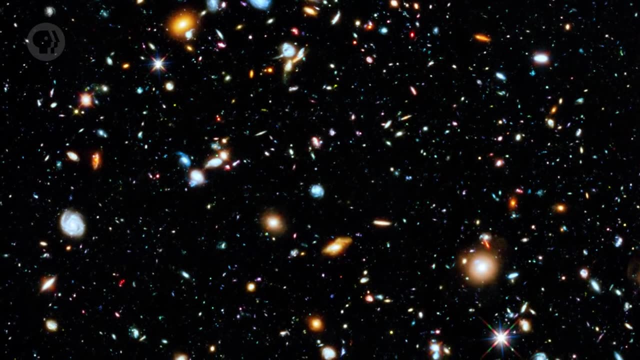 We can visit other worlds and send the pictures and data back home, or put observatories like the Hubble Space Telescope into orbit around the Earth and have it peer into the vast depths of the universe. I would argue that the past century has seen a revolution in astronomy every bit as important. 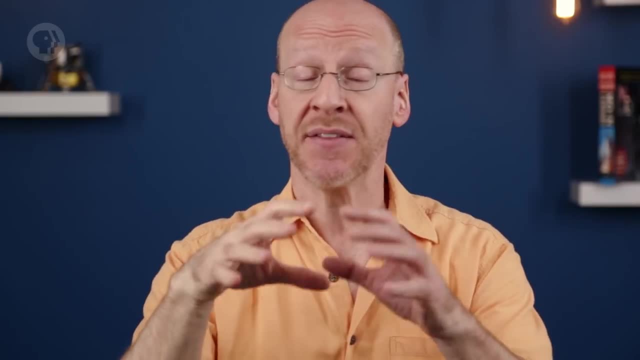 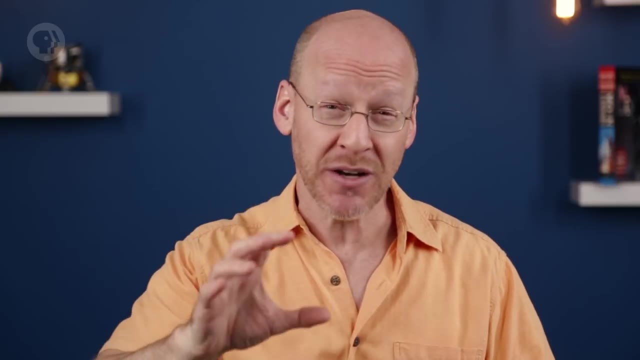 as the invention of the telescope in the first place. In the early 17th century, the entire sky was new and everywhere you pointed a telescope there was some treasure to behold. But with our huge telescopes and incredibly sensitive digital eyes now that's still true.